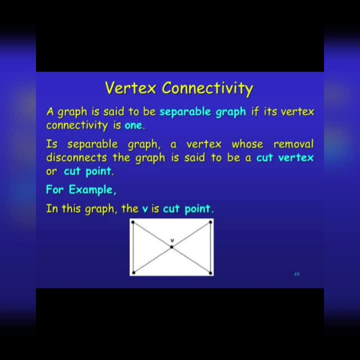 this figure Here we have marked a vertex v here. If we remove this particular vertex from this graph, what will happen? what will happen? So the edges, associated edges, incident with this vertex also will be removed. So we will get barely two components out there in this graph. that is, graph goes disconnected. 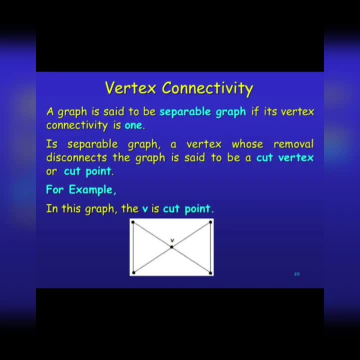 So this particular vertex is known as cut vertex. So if my particular graph has cut vertex or my vertex connectivity 1, that particular graph is known as separable graph. So vertex connectivity is actually what is? that means The minimum number of vertices whose removal becomes the graph disconnected. 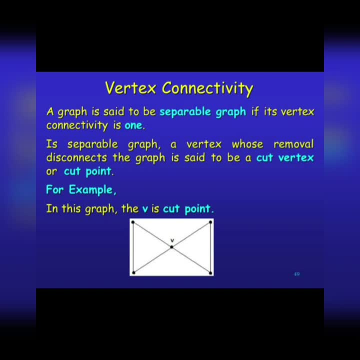 In this graph we need badly only one vertex to make this graph disconnected. So this graph has vertex connectivity 1.. So if vertex connectivity is 1, that particular graph is known as separable graph. So in separable graph, a vertex whose removal disconnects the graph which is said to be, 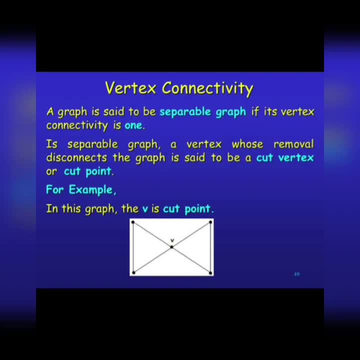 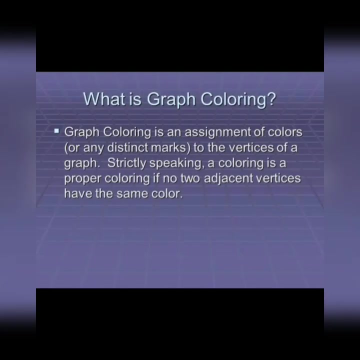 a cut vertex or a cut point. So in this graph, if we remove V means we will get barely two components out there in this graph. So V is known as a cut vertex and this particular graph has vertex connectivity 1 and which is known as a separable graph. 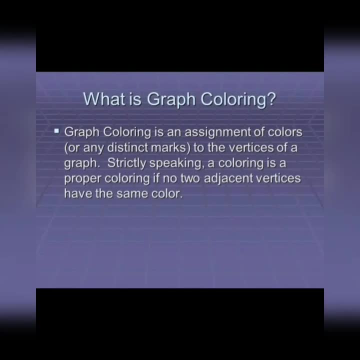 Graph coloring. this is one of the very beautiful topic in graph theory. So what does this mean? Coloring of graphs? Coloring of graphs is simply assigning colors to the vertices of the graph. Okay, graph coloring is the assignment of colors or any distinct marks to the vertices. 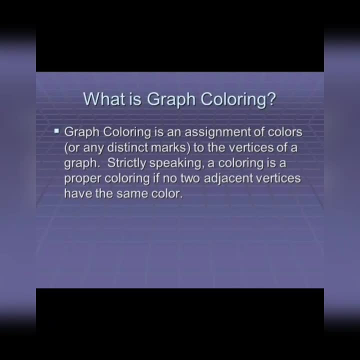 of the graph. Strictly speaking, a coloring is a proper coloring if no two adjacent vertices have the same color. So we need to color a graph in such a way that adjacent vertices are not the same. So we need to color a graph in such a way that adjacent vertices are not the same. 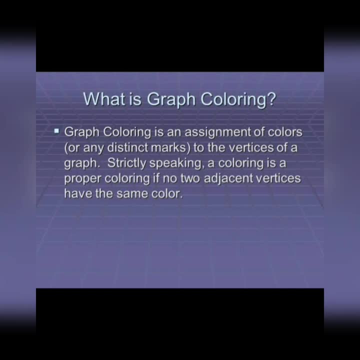 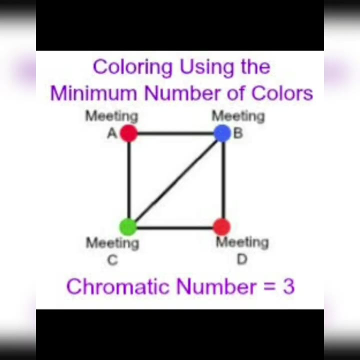 vertices are colored differently. so that is what meant by a vertex: coloring of a graph. so next is coloring using the minimum number of colors. so we cannot color a graph like that. we need to assign certain rules in that, okay, so how to color a graph, i told you before, like adjacent vertices.